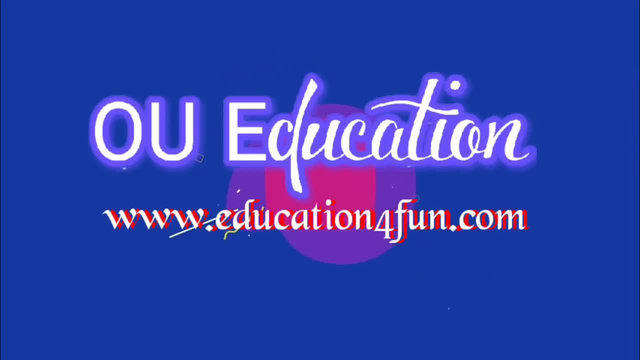 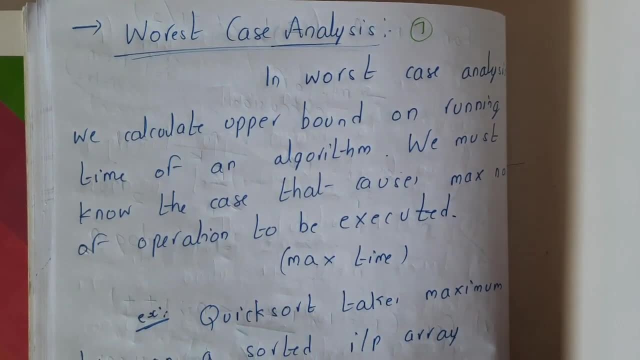 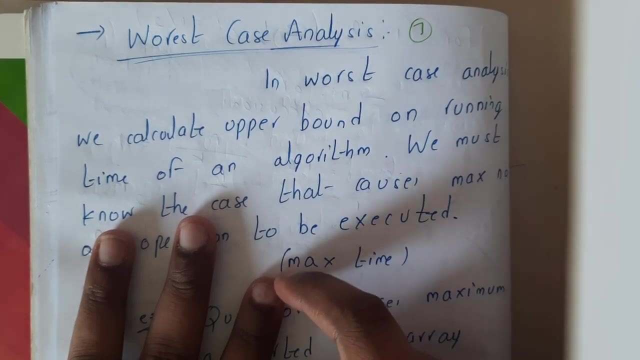 Hello guys, we are back with our next lecture. In this lecture, let us go through the three main cases in which every one will be considering right. So whenever you write an algorithm, you will be checking the best case, worst case and average case. So these are the three cases. 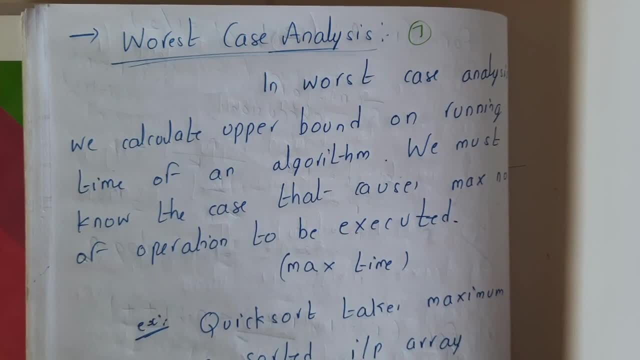 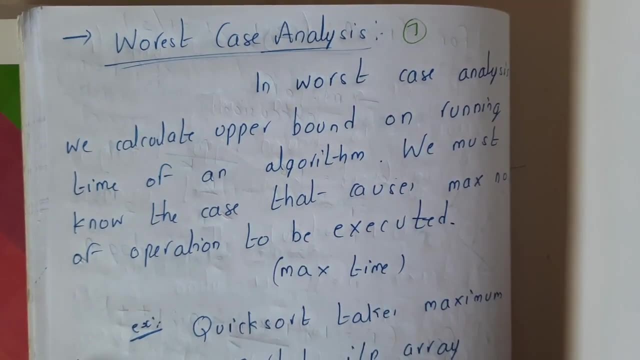 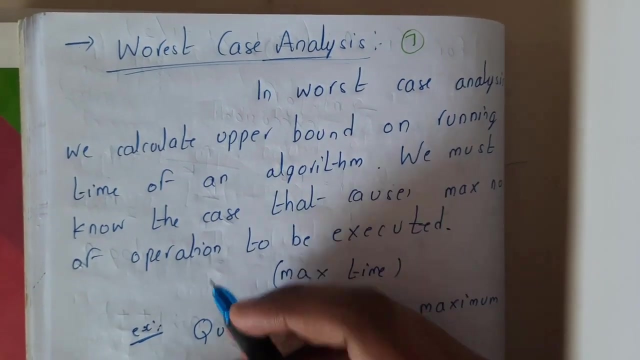 which we will be considering for any algorithm which you or anyone writes, okay? So, basically, the first thing that you should know is what is meaning of these each terms, okay, Okay. so first let us go through worst case, So, worst case. so everyone knows that. what is meaning by? 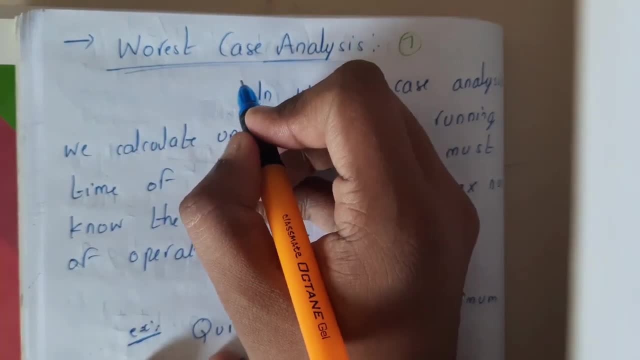 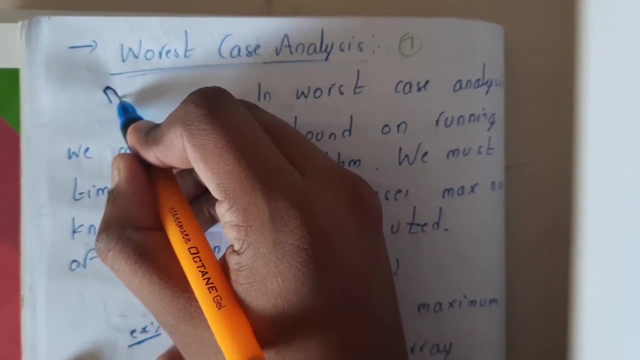 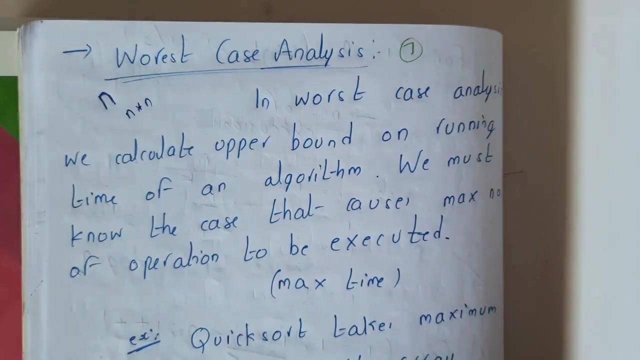 meant by worst, worst case in analysis. So basically, when an algorithm is running, if it takes n steps for every value, okay, But for some values it will be taking n into n times n steps. So I told you right, It is nothing but the free. 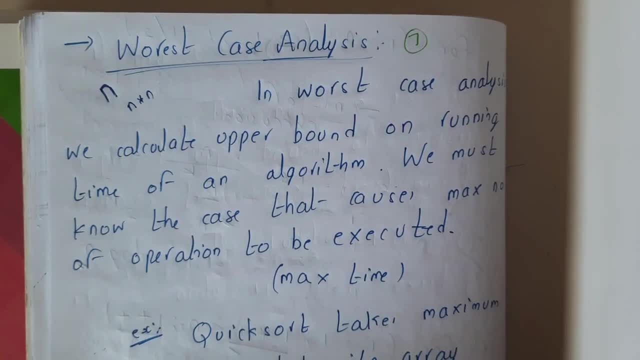 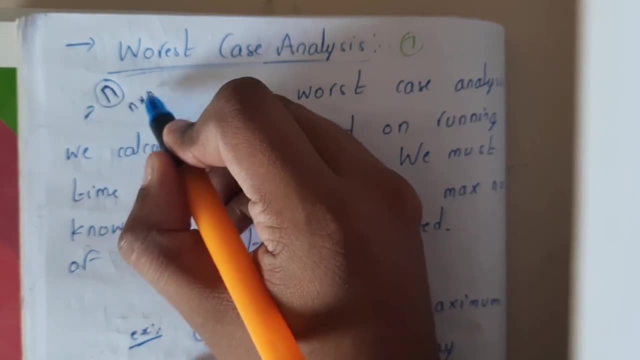 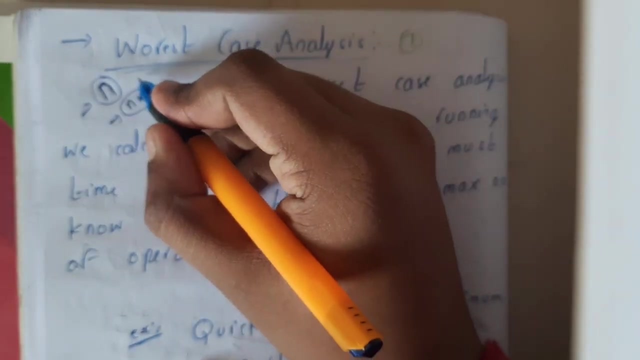 It is the frequency count which we will be using in time complexity. okay, So assume that an algorithm takes n times in the best possible scenarios and it takes a long time. that is nothing but n square in worst situations And it takes normal times. the average will be 2n. 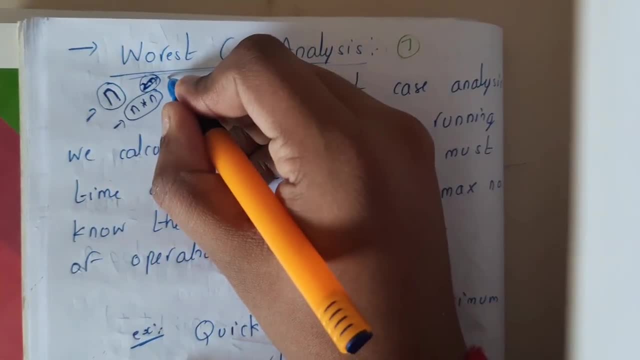 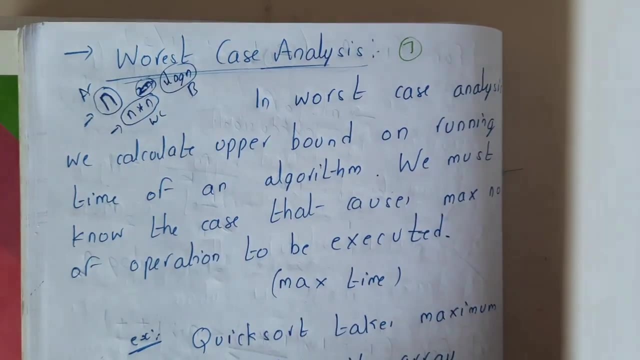 assume in that way. So 2n will not be considered, guys, sorry for that. So assume that the best case is log n, best case, average case and the worst case. So these are the three cases which I have wrote. So just for explanation, I have just wrote them. That is just an example, okay. 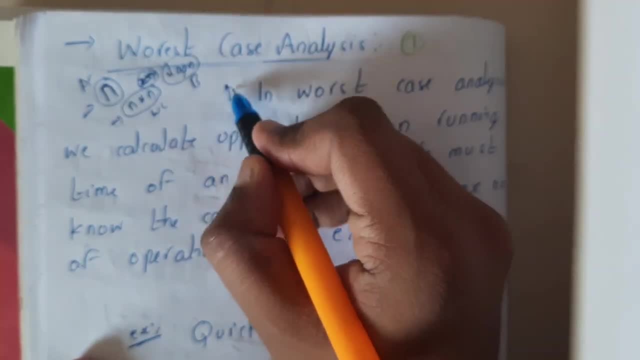 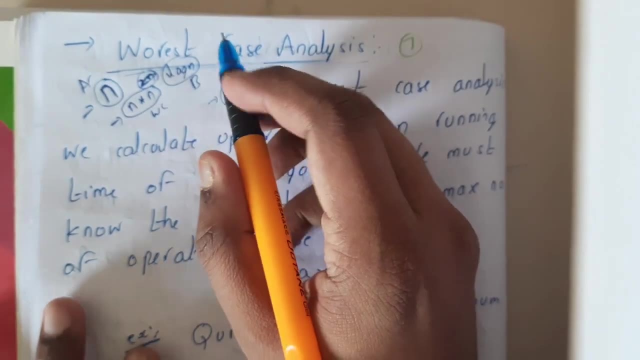 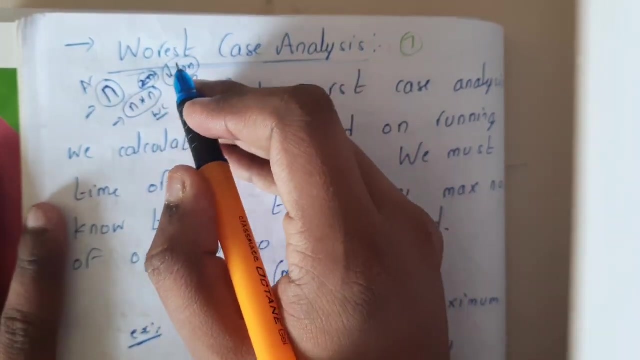 So worst case is nothing but the longest time it will take guys for a particular input. So what is the worst case of the algorithm? So it should take at max this time. for whatever input you give, it should not cross that n square complexity or n square time of that particular algorithm. okay, 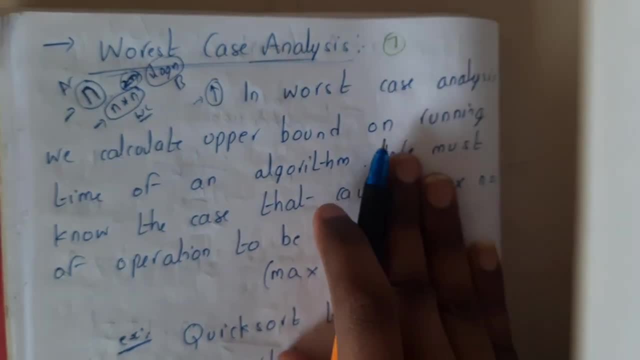 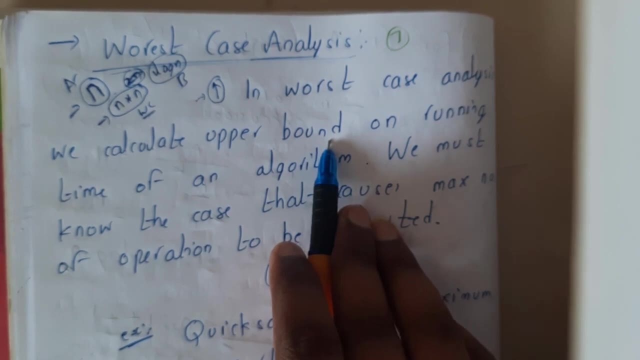 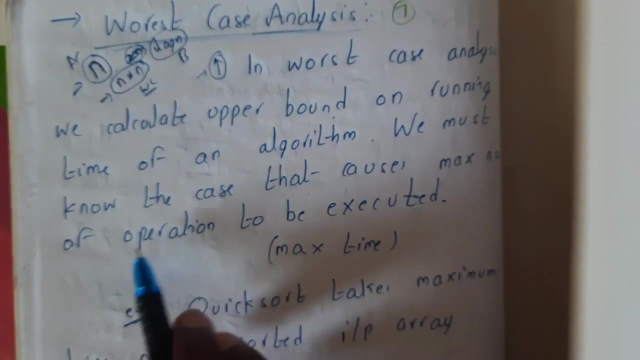 So once we are going to the definition, it will be more clear. I think so. Okay, so in worst case analysis, we calculate the upper bound. So upper bound is nothing but the maximum time taken on running time of an algorithm. We must know the case that causes the maximum number of operations to be. 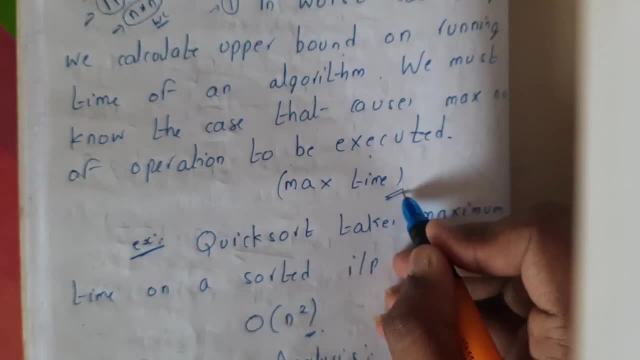 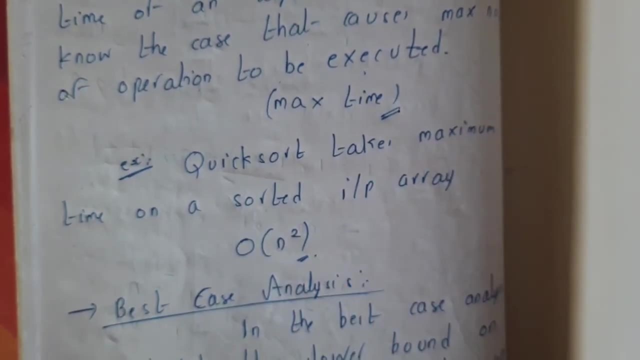 executed. That is nothing but the worst case. you can simply say that it is maximum time, Okay. so if you take a small example, I hope everyone knows the quicksort right, Okay? so we'll be discussing about quicksort in detail, don't worry about that. So I hope everyone have at least an idea about 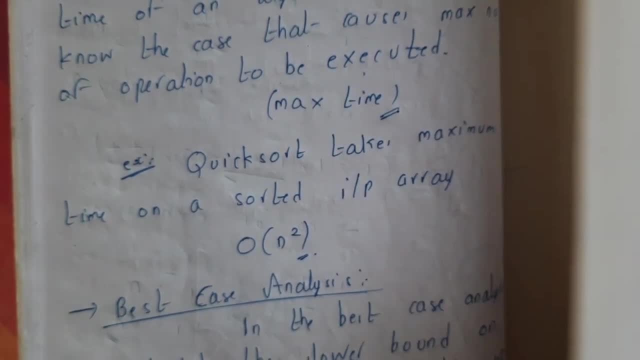 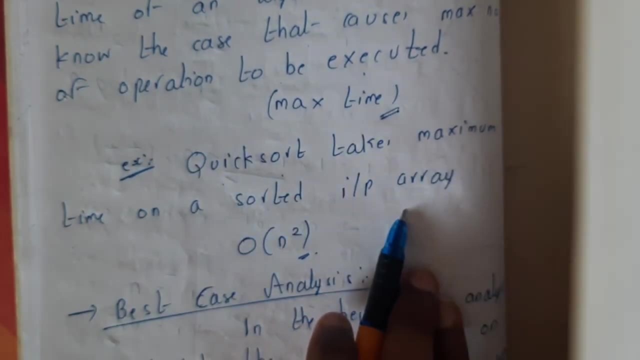 quicksort And it is a sorting algorithm so it sorts elements. okay, So quicksort takes maximum time. on sorting input array, on sorting a sorted input array. So basically, if you give a 1,, 2,, 3,, 4, and if you ask. 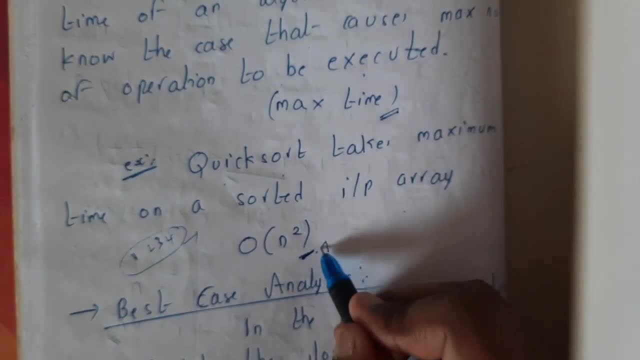 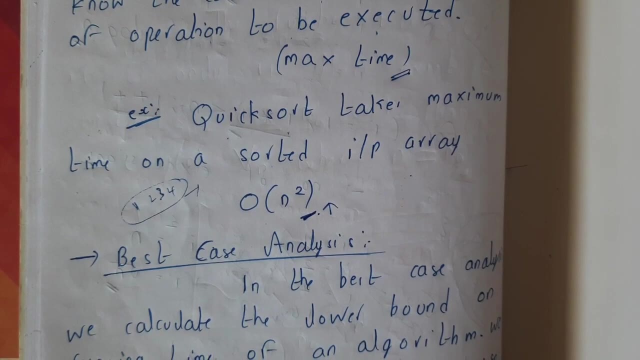 quicksort to sort it, it will take n square time, the most time it will be taking in that case of situation. So, basically, sorting algorithms are designed for sorting elements but not to sort the sorted elements right. So that is the reason why it will be checking everything. 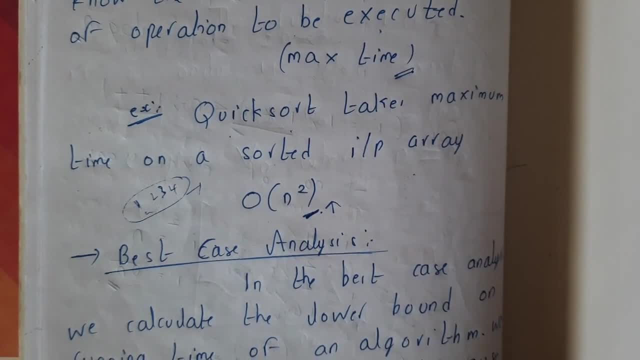 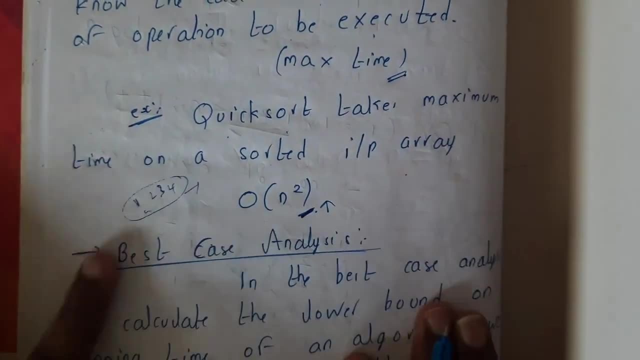 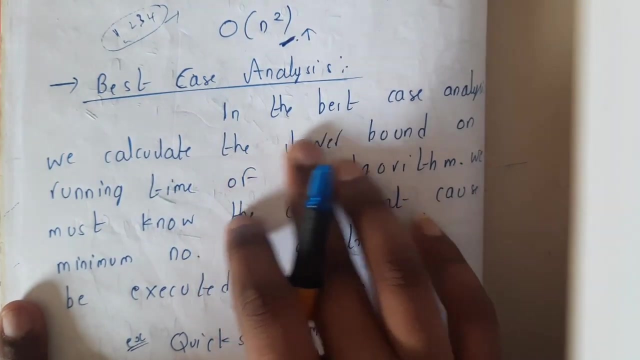 will be making the same list again by wasting some time. so this is a worst case in case of quick sort. so the longest time- remember worst- means maximum time, that's it best case. now, once you identify, worst case is maximum time, best case is minimum time, that's it. so in the best case, 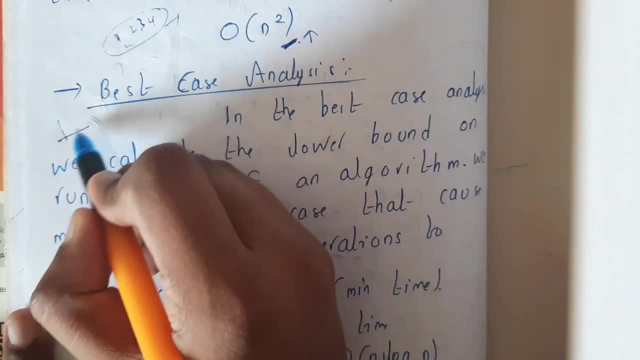 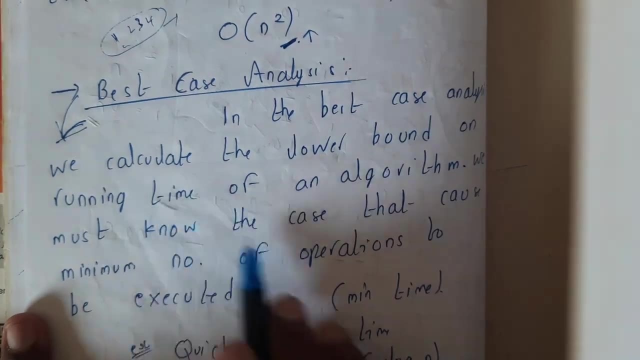 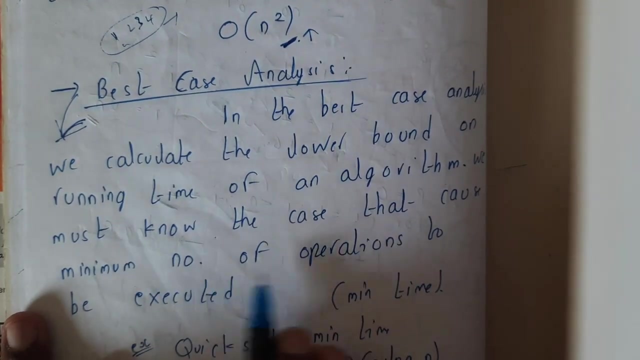 analysis, we calculate the lower bound. so this is nothing but the least time taken so previously. this is the worst case and this is the least case that is best case: lower bound- running time of an algorithm. we must know the case that causes the minimum number of operations to be executed. 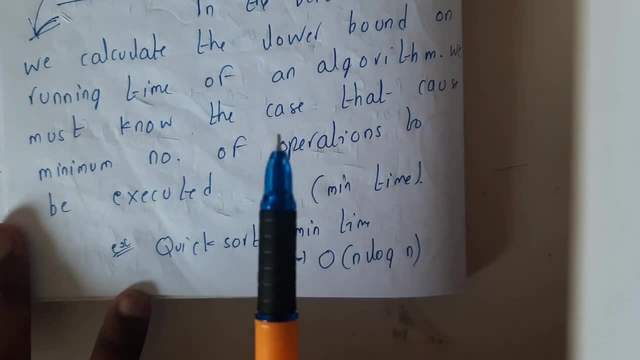 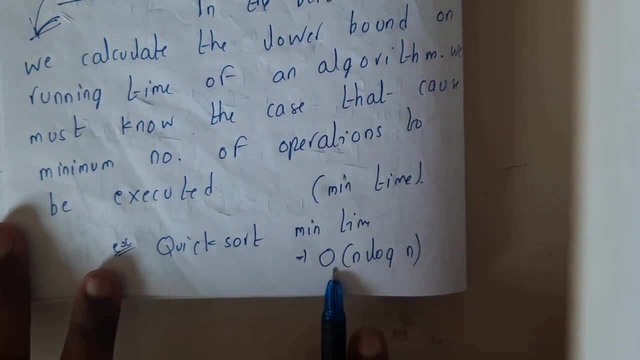 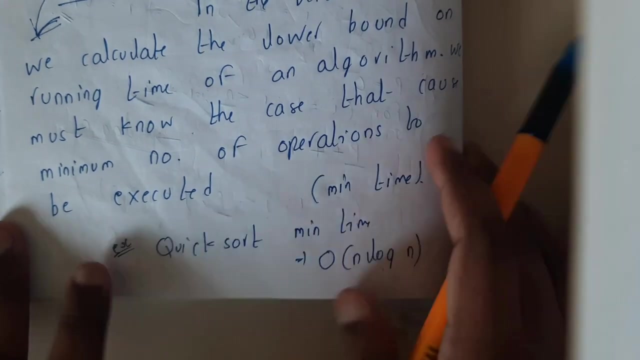 so basically, quick sort. we learned about quick sort right there. it took n square time when we gave a sorted array. basically, when you give a normal array which need to be sorted, it will take big of n log n time. okay. so, even though it is a bit lengthy, a bit long time, but it will be. 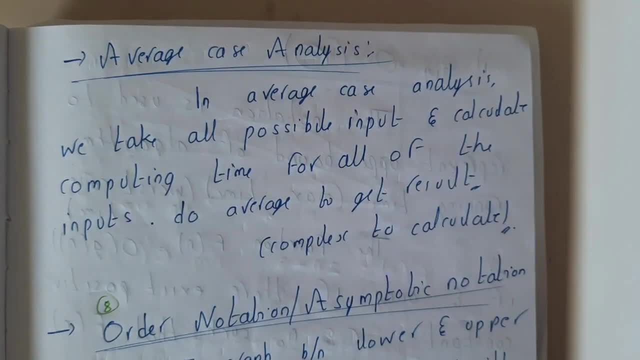 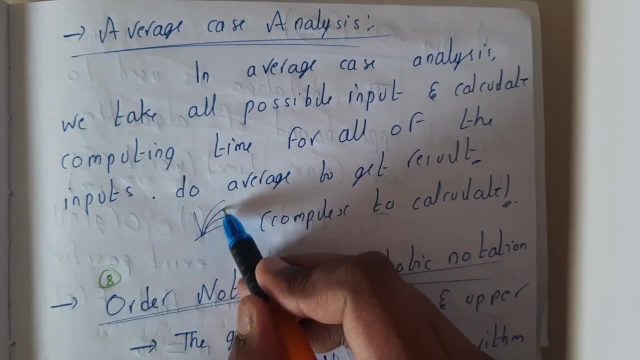 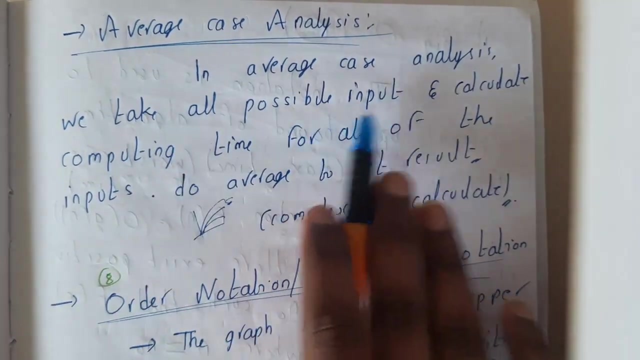 in that time. okay, so average case. so basically, average case is nothing but in between both of them. so basically, if both of those are there like that, it will be in between them. so it is nothing but the average case of those both. you can say simply: so in average case analysis we take all possible inputs and calculate the